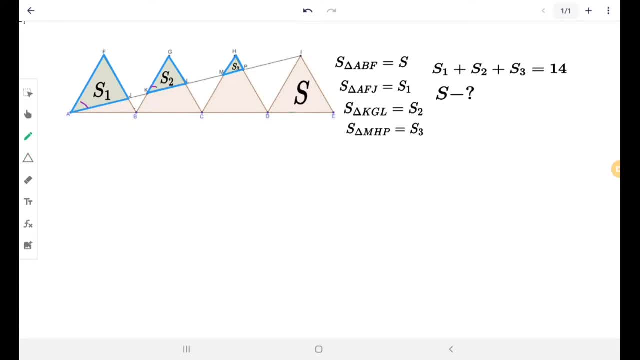 The angles FAJ, GKL and HMP are equal, as they are corresponding angles. Angles AFJ, KGL and MHP are equal, as they are corresponding angles. These are angles of equilateral triangles, So the triangles AFJ, KGL and MHP are similar. 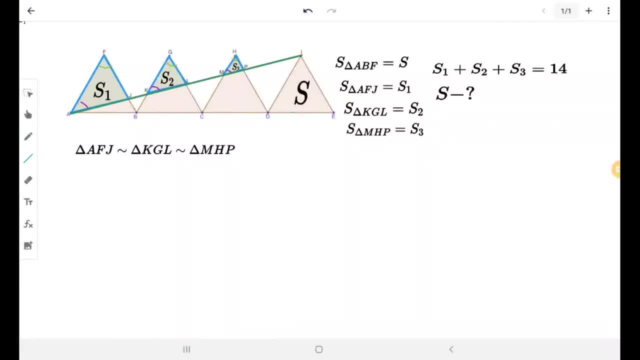 According to Thaley's theorem, if angle IAE is intersected by parallel lines FB, GC, HD, IE and one of the lines is split to equal segments AB, BC, CD and DEI, and one of the lines is split to equal segments AB, BC, CD and DEI. 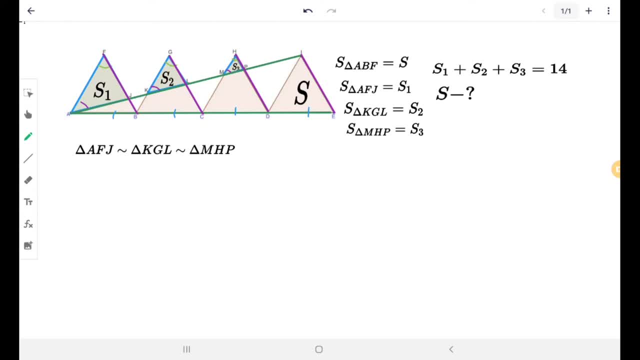 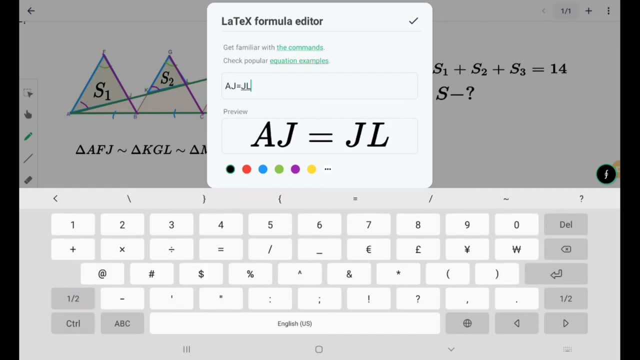 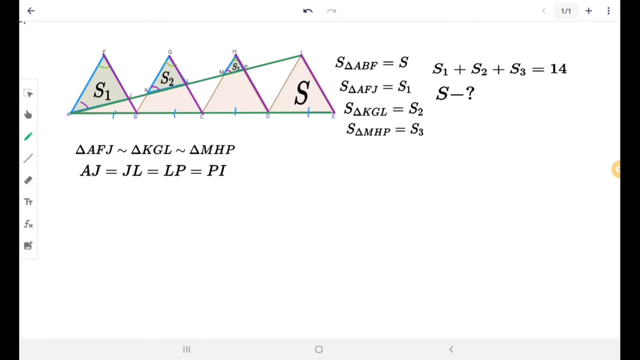 then the other line, AI, is also cut into equal segments, which means that AJ is equal to JL and is equal to LP and is equal to PI Angle. IAE is also intersected by parallel lines GB, MC and ID, so AI is divided into equal segments. 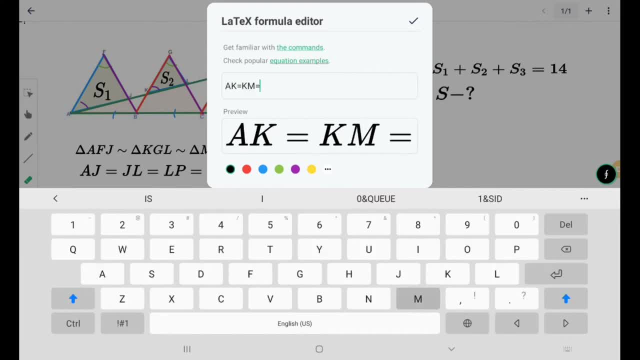 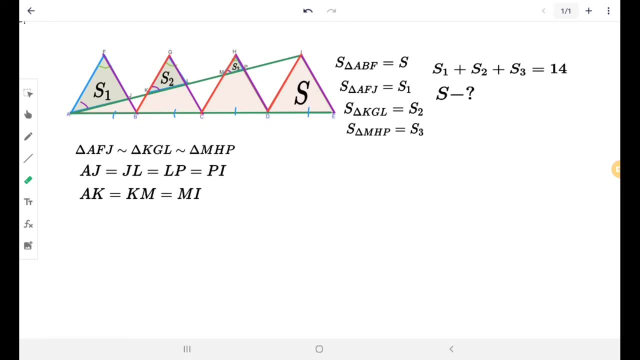 AK is equal to KM and is equal to MI. Using these equalities, we can get that AJ is equal to PI and JK is equal to MP and KL is equal to LM. This means that the triangles AFJ and PDI are equal because of one equal side and two equal angles. 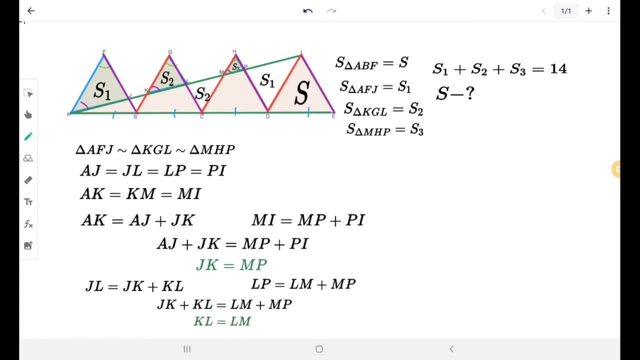 This means that the triangles AFJ and PDI are equal because of one equal side and two equal angles, Just as the triangles KGL and LCM are equal and the triangles MHP and JBK are equal as well. The equations we have bring us to the proportions between the AJ, KL and MP sides. 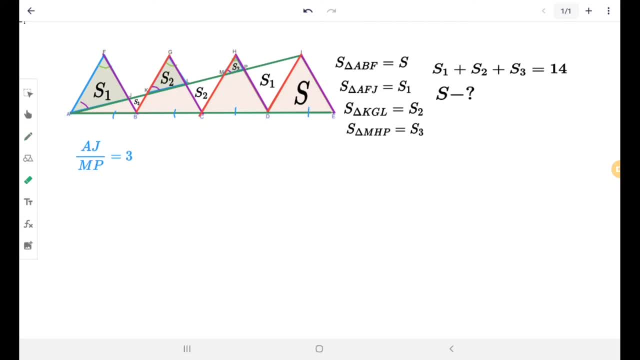 This proportion could bring us to the similarity ratio of the sides of AFJ and MHP triangles. This proportion could bring us to the similarity ratio of the sides of AFJ and MHP triangles. Then the ratio of the areas of these triangles is the square of the similarity ratio of their sides.